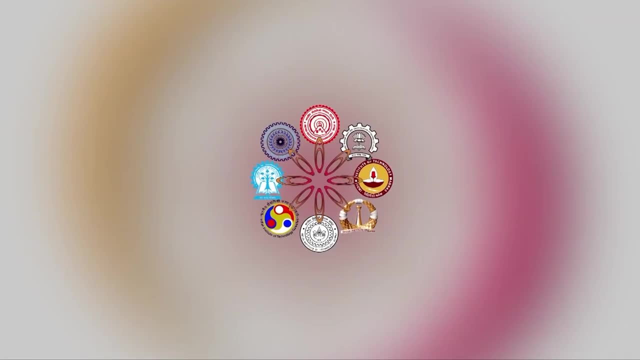 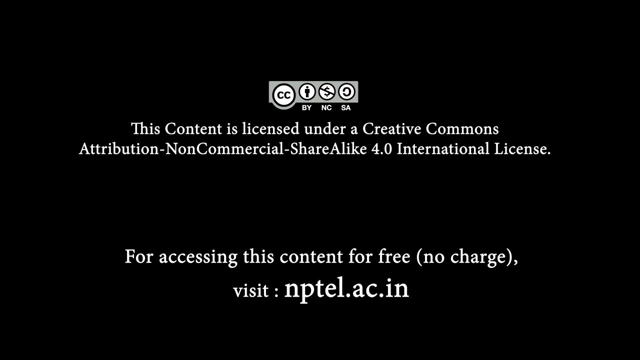 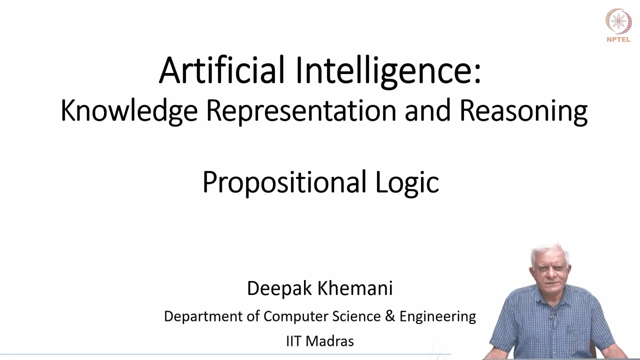 So we have been looking at logic in general. We have not yet defined the language. We have assumed that we have some language in which there are sentences- alpha, beta, gamma and so on- And we have looked at the fact that you can create more sentences or compound. 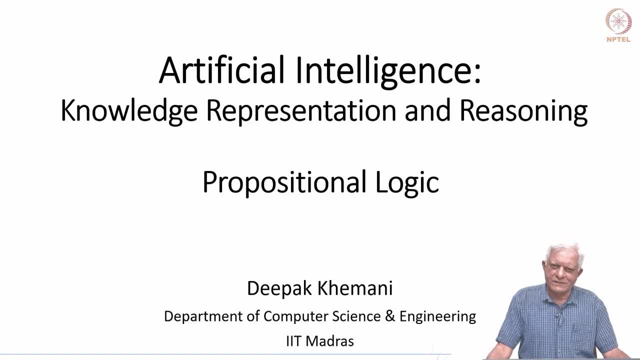 sentences using the logical connectives. So we saw a set of connectives, One unary connective, which is the negation, and we saw a few binary connectives which take two sentences and produce a new compound sentence. And then we did a little bit of analysis to see that. 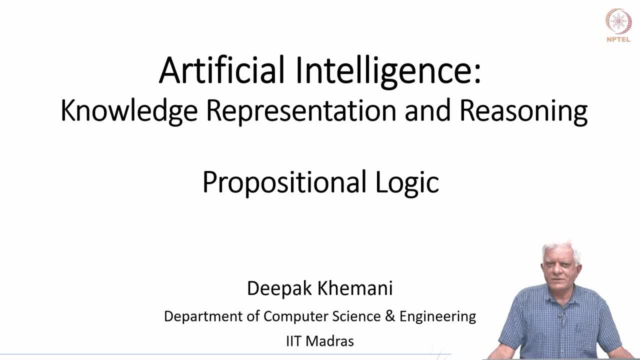 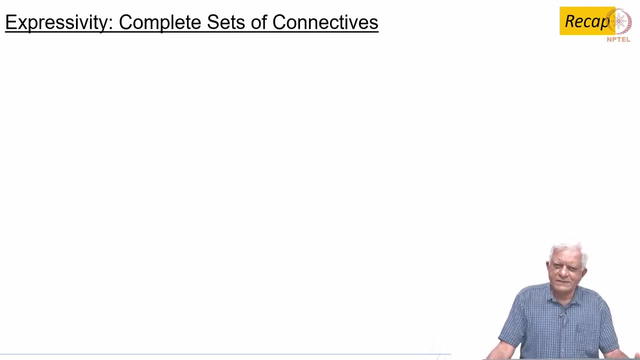 of all the 16 possible binary connectives, how many do we really need essentially? And we saw- and maybe we will begin with that today- that a small set is necessary. So let us look at that essentially. What do we mean by a complete set of connectives, Basically? 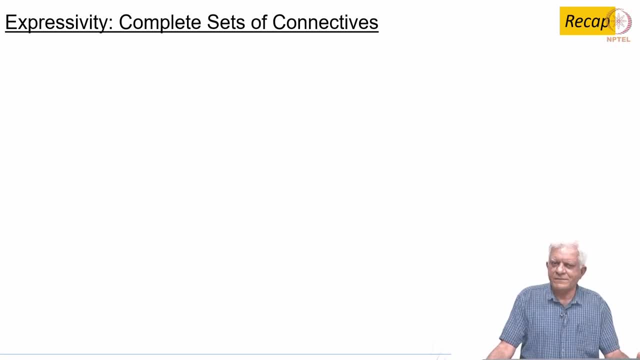 whatever can be expressed in whatever language we are defining, and today we will define our first language, which is the propositional logic That whatever can be expressed in that, in that language, using all connectives, what is the minimum set that you can use, or what is the sufficient set that is enough to express? 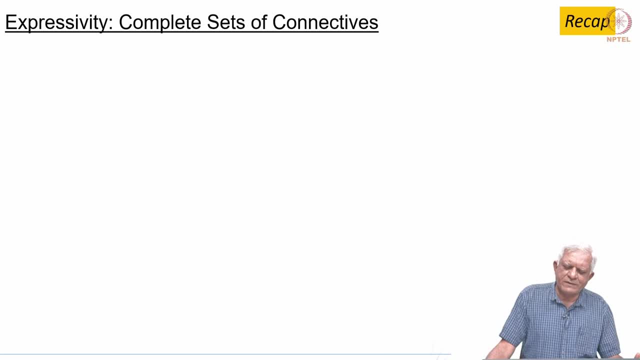 everything that can be expressed. So that way we do not have to work with all the connectives. And we saw 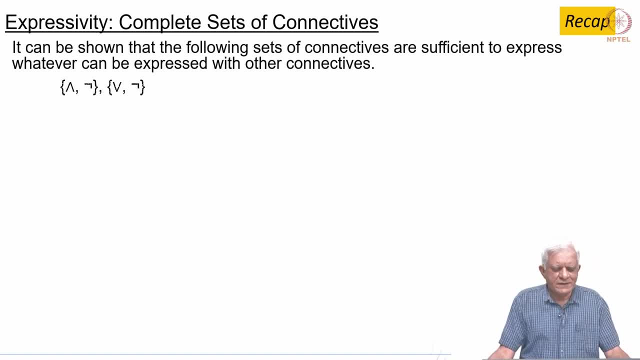 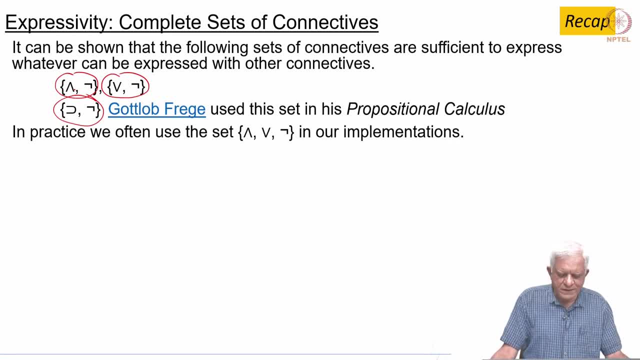 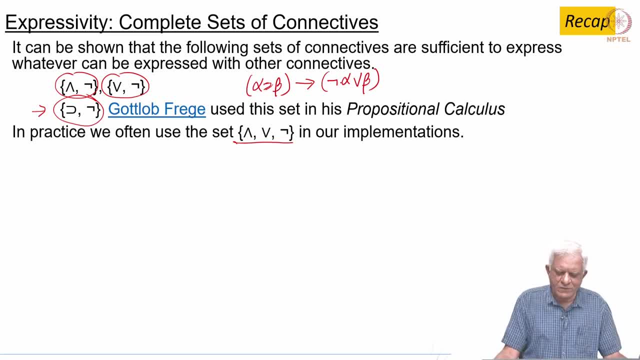 can represent in this that particular language using only these connectives, and we do not need the other connectives. The expressions that we use may be longer. in this case, the length is the same, more or less, in the sense that we have one connective is replaced by. 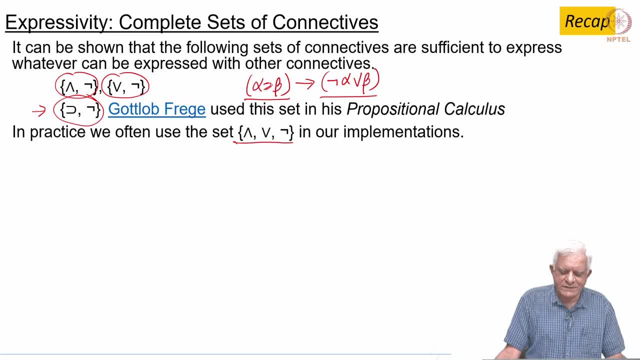 two connectives, but one of them is the unary connective, but for other cases it may be different. So for, as an exercise may be, you should try to express this using only let us say or and not, and see how that can be done essentially. So you will see that the size 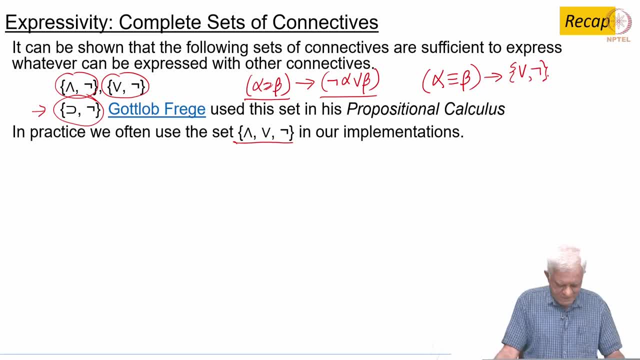 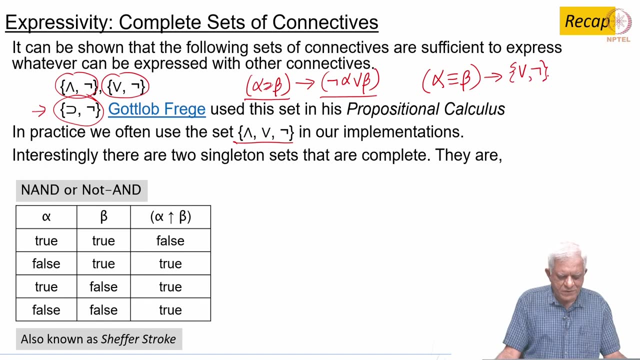 of the expression is different, So the initial step increases essentially. We also mentioned in passing that there are some singleton sets which are complete, and one of them is the nand, which is same as not, and, And we had seen that you could also write. 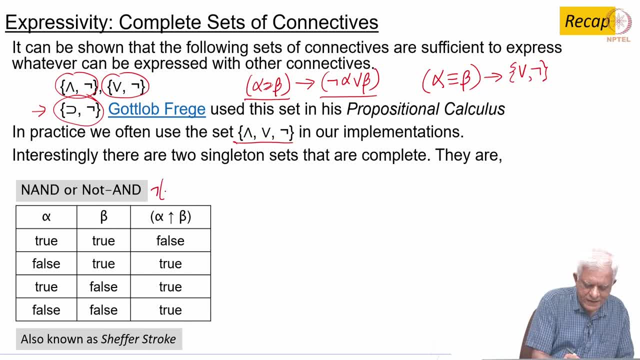 it as not of and and and would be, in this case, alpha and beta. So, but instead of athletes, of calling it not and, we are calling it nand, which, and we are using one symbol to do that essentially, And this symbol is that arrow pointing upwards which is also called Schaefer's. 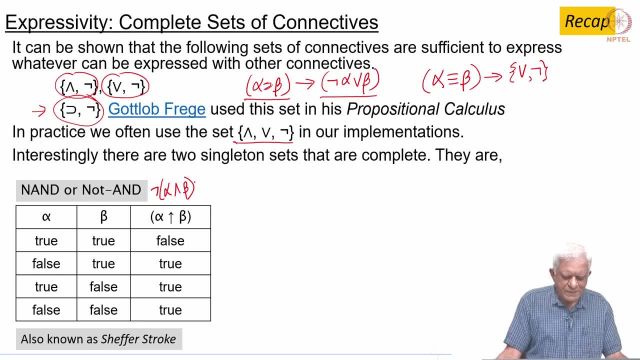 stroke and you can see that the truth values are opposite of that of and. So if I write the truth values of and here try to squeeze it in, So and will be true only when these two are true and in the other cases it will be false. And you can see that the relation 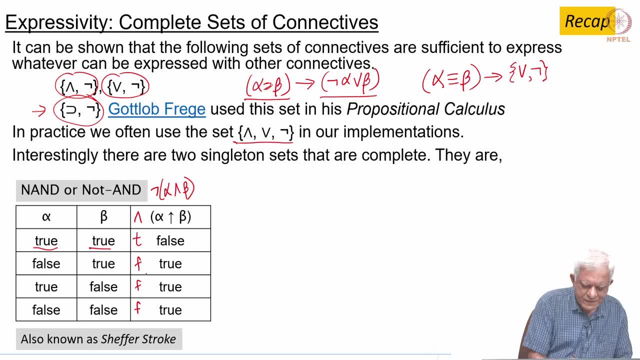 between true and false is the same, that it is, that at every row it is the negation of the other. So it is so. so nand is nothing else, but not and. but the interesting thing about nand is that anything you want to say in that language, you can say using only this: 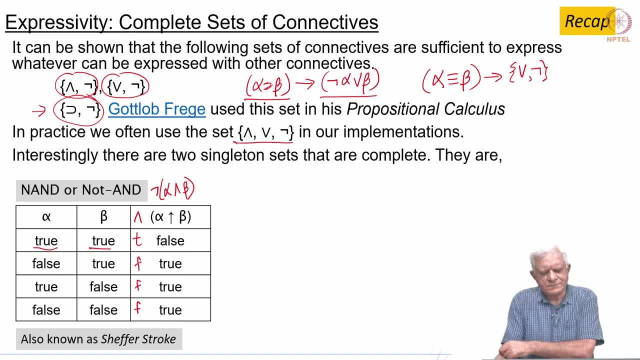 nand connect connective. It has implications in building circuits because logic circuits are essentially hardware implementations and then if you can use only that one one, one gate- nand gate as it is called- to implement the circuit, then you know life has certain plus points there, essentially. 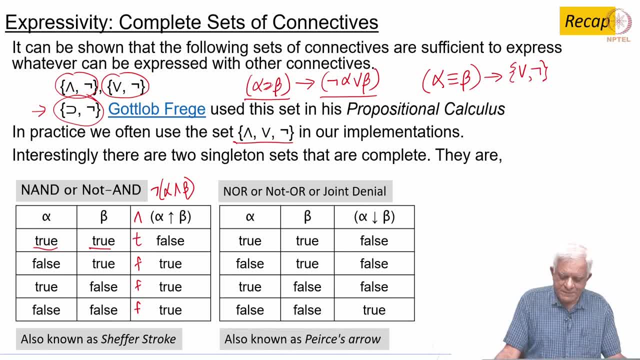 Another connective, which is also complete by itself, is the NOR gate, or NOR logical connective, also known as joint denial, also known as Pierce's arrow. So these are the logicians who, you know, wrote about these connectives. By joint denial. we mean what, We mean that. 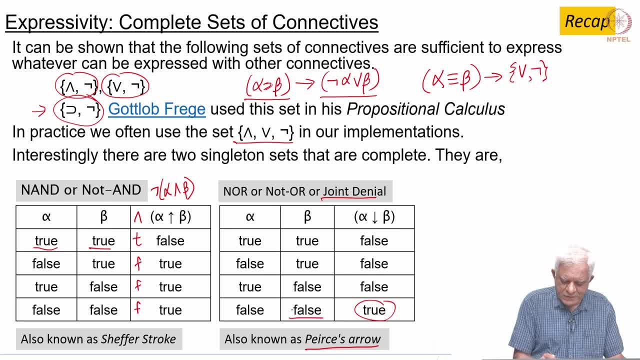 the sentence will be true only when both alpha and beta are denied essentially, That alpha cannot be true or and beta also cannot be true. So both must be false essentially, and only then this is true essentially and you can work it out that this is the same as not alpha or beta. So by now you should. 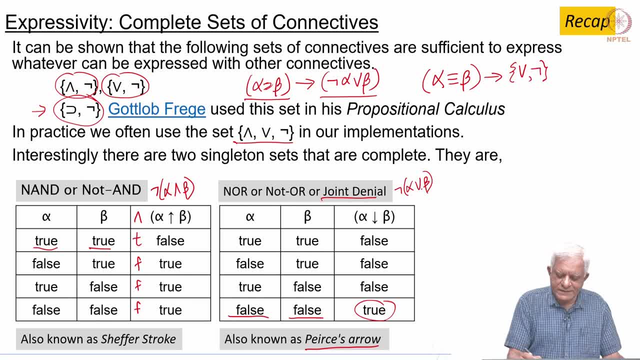 have got the hang of the language. You can see that this expression, which is not alpha or beta and the brackets are around alpha or beta- is not the same as this other expression where it is not alpha or beta, and they are entirely different essentially. So that is. 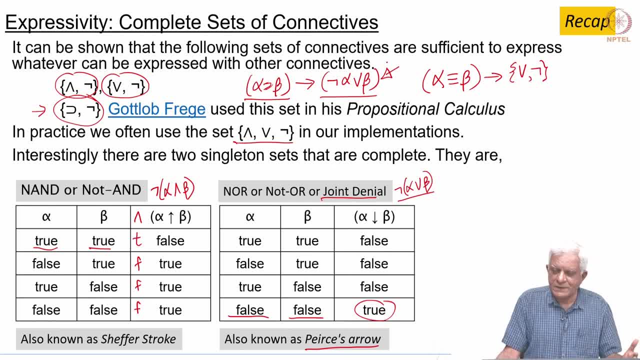 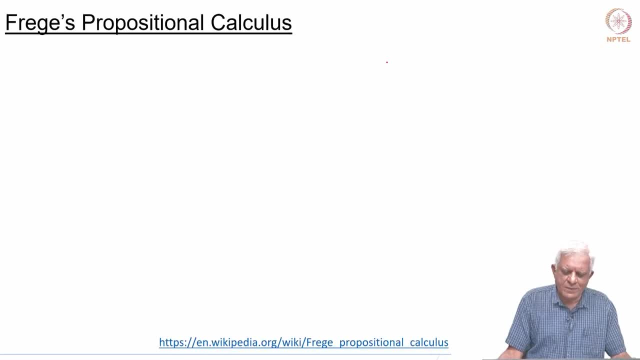 one of the differences between formal languages or formal logics and natural languages. So in English, of course, we can go on rambling so on, but in logic you have to be very precise. So let us talk about this, Chege's proportional calculus, The other issue that we want to. 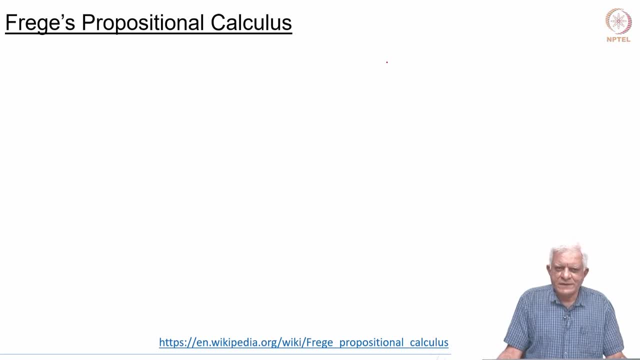 look at very briefly is that of doing logical inference. So, if you remember, the way that logical inference works is that you have a set of rules of implication. We saw a few of them: modus ponens, modus dolens, disjunctive syllogism, hypothetical syllogism. 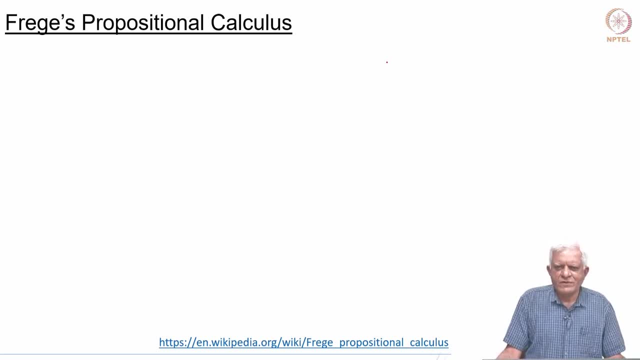 conjunction, addition and all of these. essentially What they allow you to do is to add new formulas to the knowledge base. So it is so. that is the proof process is an entirely syntactic process- that you look at a pattern and you can add something new to that. essentially, 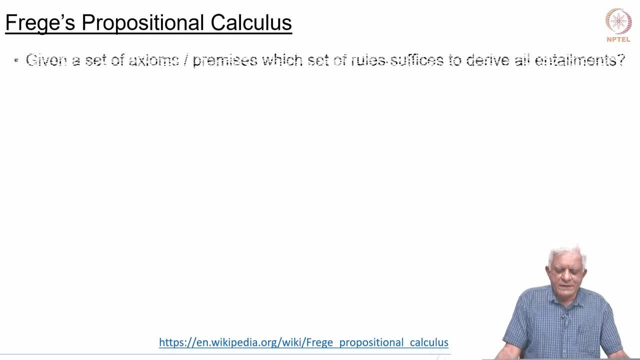 So what Chege showed was that just one rule of inference is enough for completeness. So this is a different notion of completeness. When we talked about completeness of the connective we say we were talking about the completeness in terms of expressivity, that everything that 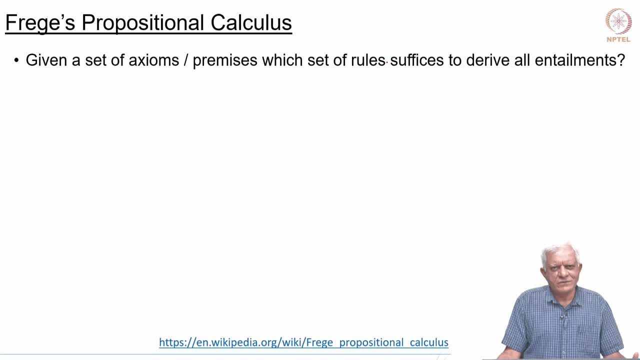 you can express in that language can be expressed using only that small set of complete connectives. But the question that we are looking at now is that what are the hardware and hardware? What are the hardware and hardware in the language? the language and the language Are there so that 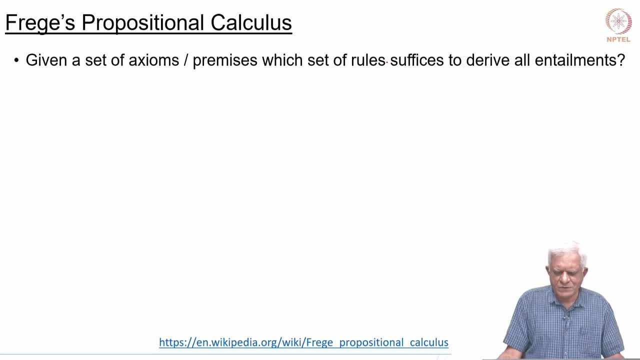 looking at now is that, given a set of axioms and premises that is given to you, which set of rules suffices to derive all entailments? Remember the notion of completeness in logic. a logic is complete if everything that is entailed can also be proved essentially So. 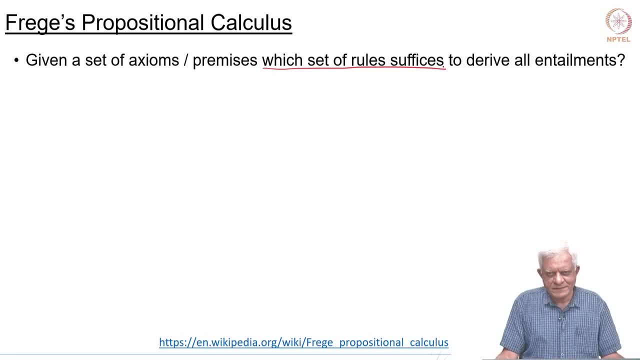 how many rules do we need to be able to do? that is the question that people have been asking since logics were devised, And what Gottlob Frege showed was that just one rule of modus ponens. So if you remember modus ponens, it says: if you are given alpha and 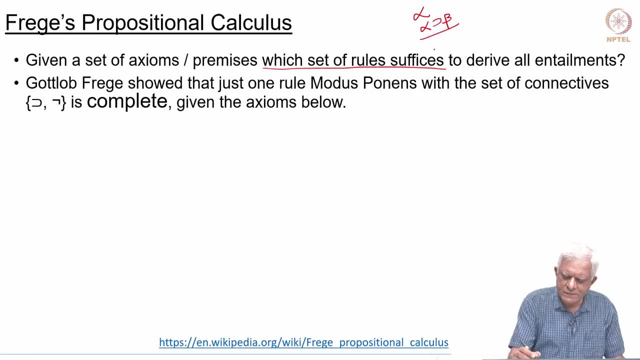 if you are given alpha implies beta, then you can infer beta, So you can put the therefore sign here. This is a modus ponens, rules of inference, that if you, if you can match alpha with something in the knowledge base and if you can match alpha implies beta with something. 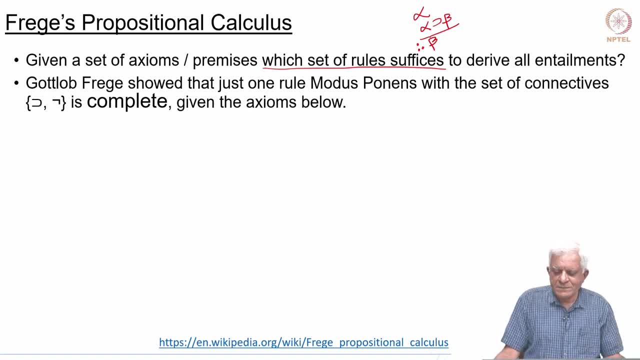 in the knowledge base. then you can add beta, So you do not have to worry about truth values and stuff like that. essentially, And what he showed was that this one rule of modus ponens, and with this small set of logical connectives, is complete, provided you accept the axioms. 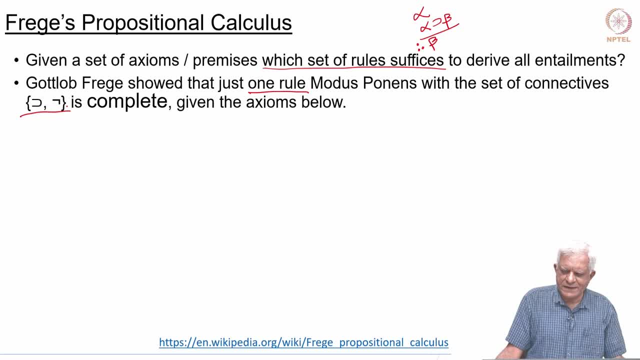 that he has specifying. We will look at this axioms in a moment. What do we mean by complete here? In the case of Frege's proportional calculus, we will see that you can derive all true statements, And when we say true statements, we mean the statements that are entailed. So his logic. 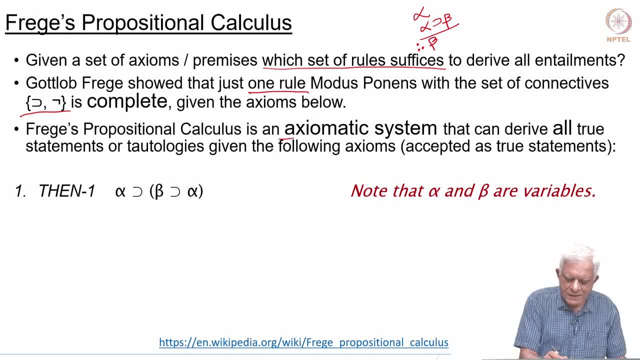 is called an axiomatic system because we start the knowledge base is a set of axioms, So axioms are basically statements that mathematicians specify and say that you accept this and everything else will follow. essentially, So this is. these are the axioms of Frege's. 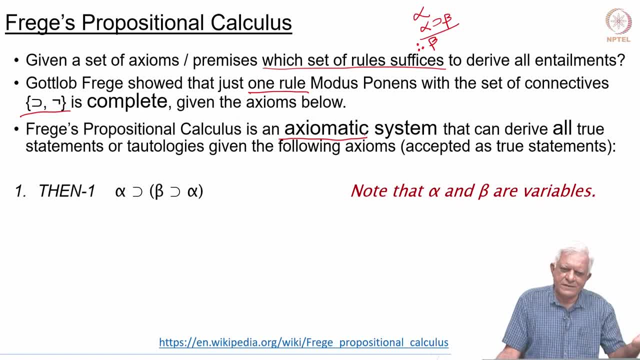 proportional calculus. Mathematicians, for example, have given a set of axioms to define number theory. I do not know. we, if we get time, we will probably look at the axioms. So we have. we have said this before that we know that. what is the notion of a number? 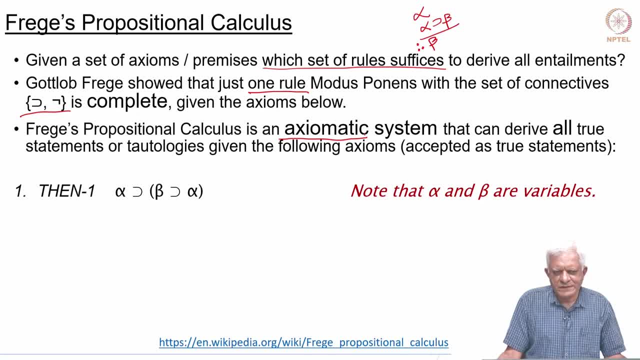 but we are not quite sure as to how to describe a number. Of course we know how to represent it using some symbol. So, for example, the number 7 we discussed- but what is a number? We will try to see sometime later- and that there is a set of axioms called Peano axioms. 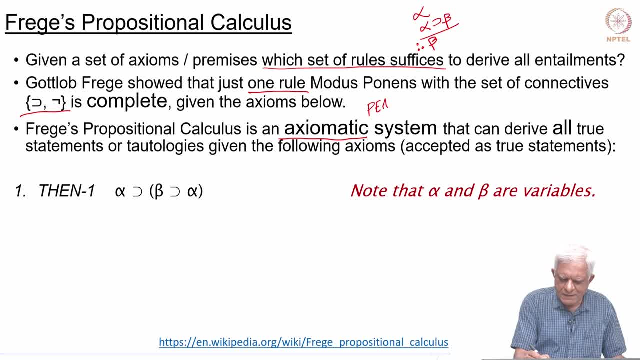 So Peano axioms. So Peano axioms, It is a set of axioms called Peano axioms- if you get time we will look at them- and they basically define number systems and on top of it all number theory has been built. 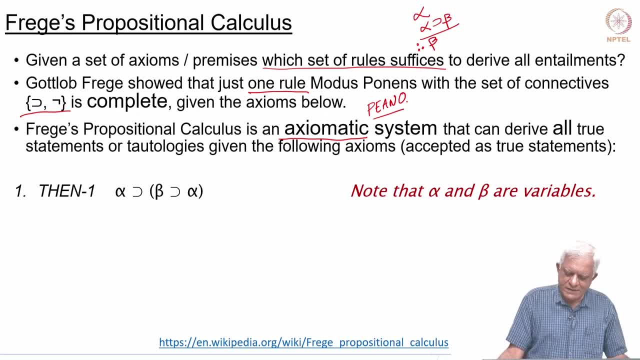 essentially So. anyway, we are talking here about logic, here, proportional logic and Frege propose a set of six axioms, and the first of them is that alpha implies beta implies alpha. So note the brackets. the brackets are, of course very important, as I said. a short 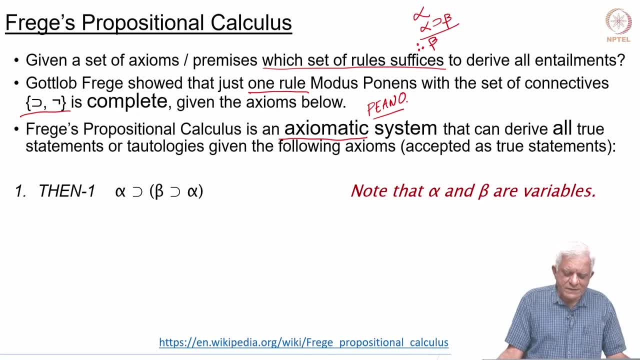 while ago. What does it mean? to say that this is an axiom? It means that this statement is going to be true. Whatever you plug in for alpha, whatever you plug in for beta, whatever you plug in for alpha and beta, there are only two things here: This statement will turn out to be true. 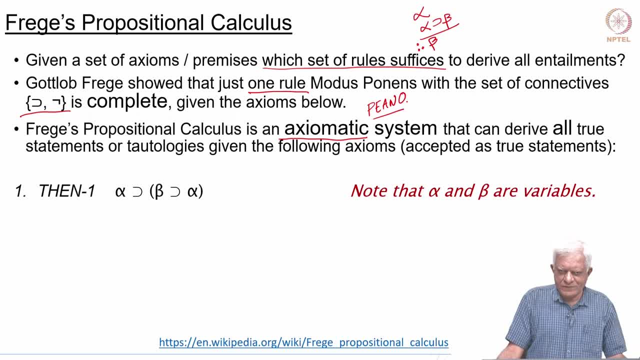 and I encourage you to draw the truth tables for all these six axioms that we are writing and make, and convince yourself that these are indeed axioms which are true. So this is called, then. one alpha implies, beta implies alpha, and we can plug in anything. 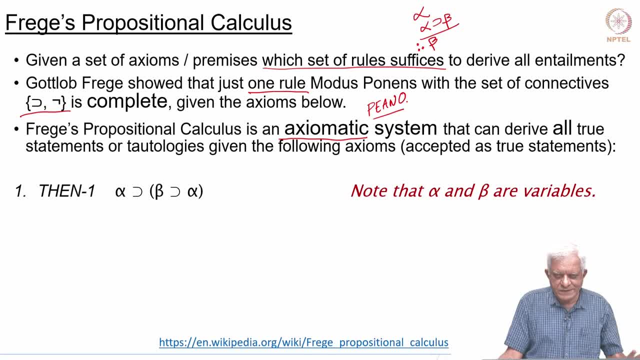 for alpha. we can plug in anything for beta. The only constraint, of course, is that whatever you plug in for the first instance of alpha, you must also plug in in the second instance of alpha, which is the normal notion of a variable. A variable stands for something else. This: 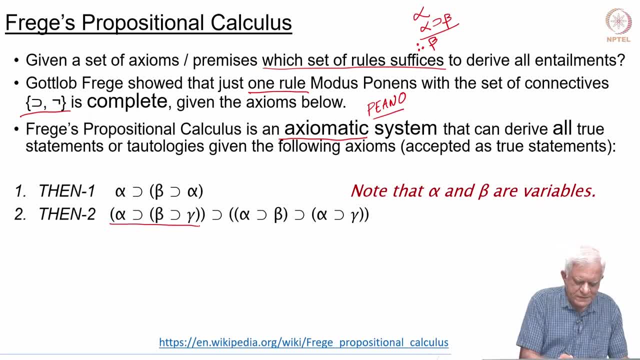 is then two. So the antecedent is this: alpha implies beta, alpha, So and it says that if this is true, then this, the second half, is true also. The difference is there is a third variable here which is not there in the first one. So alpha implies: 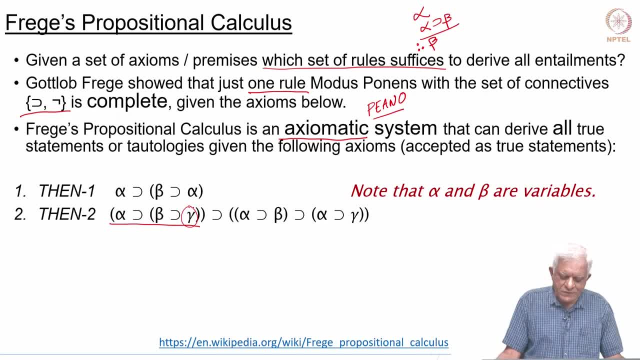 beta implies gamma. If that is true, then you can write: alpha implies beta, the whole thing implies alpha implies gamma. actually, The third axiom called then three is then this as follows: It says that alpha implies beta implies gamma is same as, not same as. 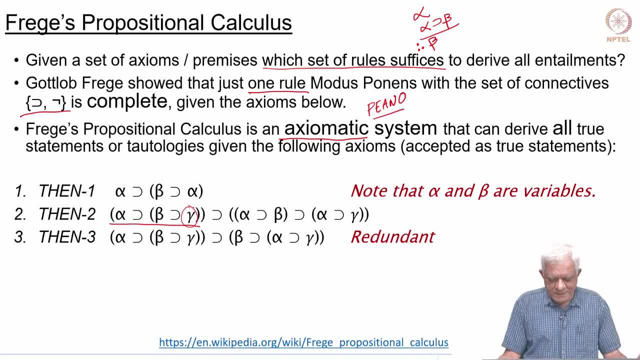 You can add: beta implies alpha, implies gamma, essentially, And it has been shown subsequently by other logicians that this is really a redundant axiom In the sense you do not really need it for completeness. even without this third axiom, the system would be complete Then. 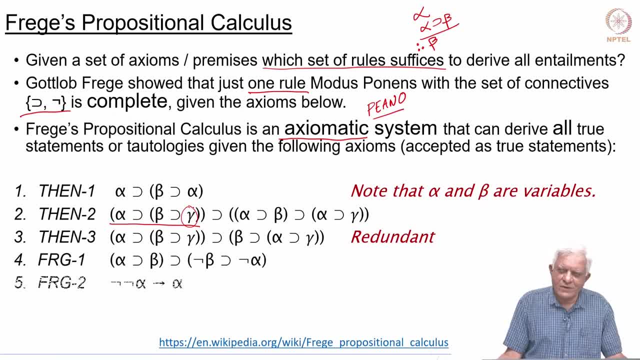 we have this. Then there are three axioms which have been called as FRG 1, 2, 3.. So FRG 1, 2, 3 is that alpha implies beta, implies not, beta implies not alpha. Again, you should construct the. 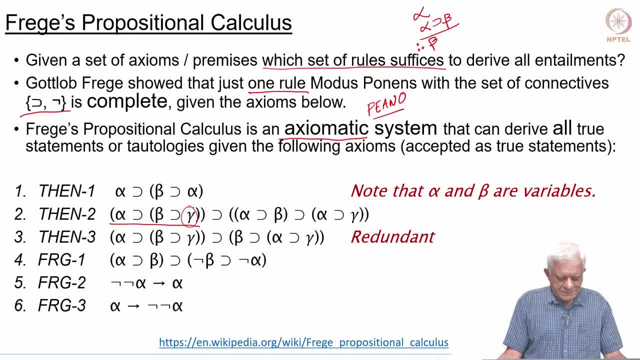 truth table to verify that this is the case. If you look at the, if you remember the rule called Modus Tollens. the Modus Tollens rule was as follows: that we are given not beta, and if you are given alpha implies beta, then you can infer not alpha. So you can see that. 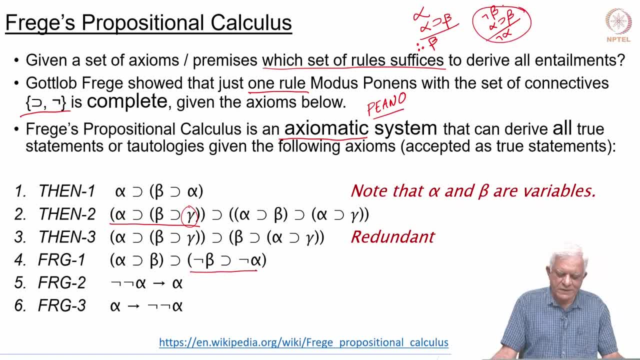 the right hand side kind of corresponds to the Modus Tollens rule that instead of alpha implies beta. you are working with not beta. If you were working with not beta implies not alpha, then this would become Modus Ponens, essentially because not beta would come here. 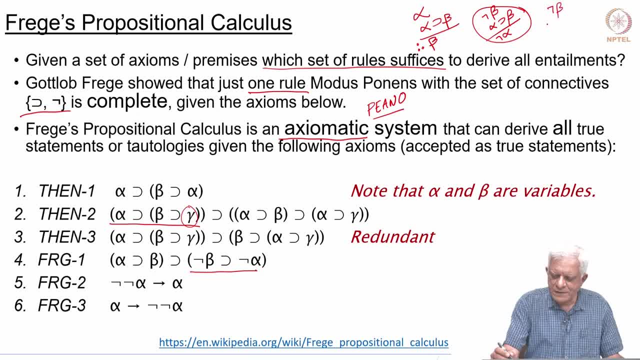 and so this would become not beta, and not beta implies not alpha, and then not alpha. That would be like Modus Tollens. So you can see that Modus, Modus Tollens, which is this one mt, is just Modus Ponens in another form. essentially, This is Modus Ponens, The antecedent. 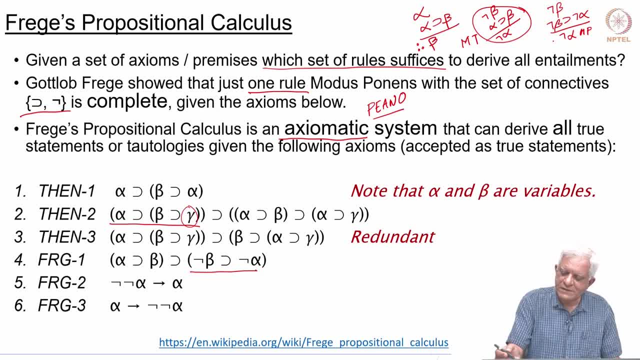 implies the consequent and given the antecedent, you assume the constant. In Modus Tollens, you would assume the negation of the constant consequent and you infer the negation of the antecedent. So it is nice to play around. 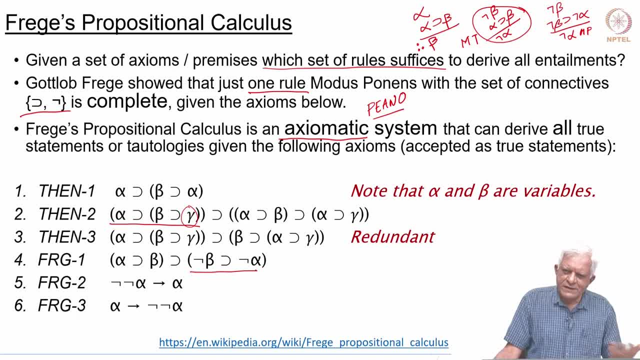 with logical systems and see that, you know, sometimes there are shorter proofs if you have more rules of inference, and that is a question which any designer of theorem proving system or a program which does proofs will have to content with. essentially, The last two are pretty obvious. as you can see, it says that the negation of negation. 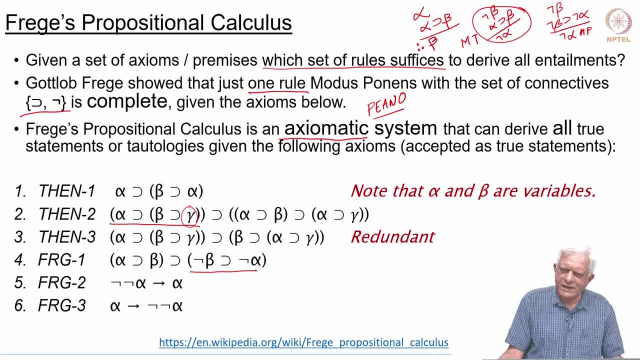 is positive. So not of not. alpha is alpha and if you remember the truth tables then you can see that that is obvious, that that, for example, if you start with alpha and then you put a not, then if alpha was true, then it will become false. you put another not and 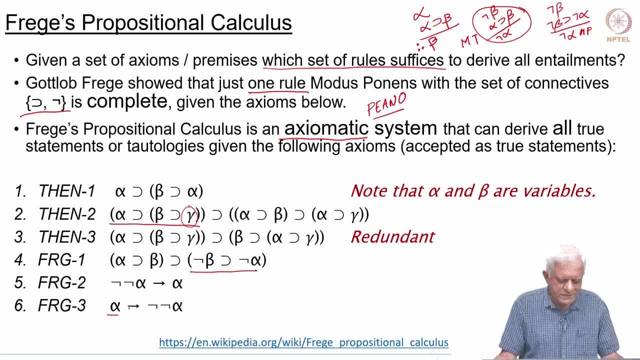 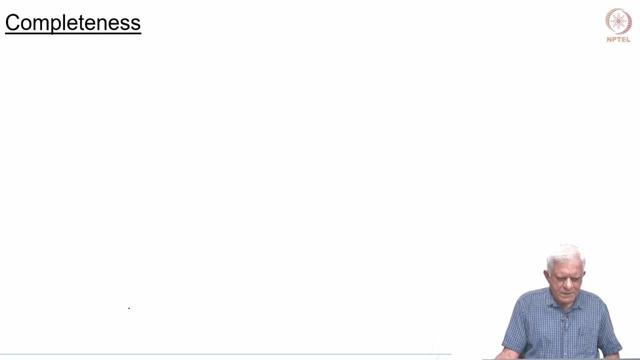 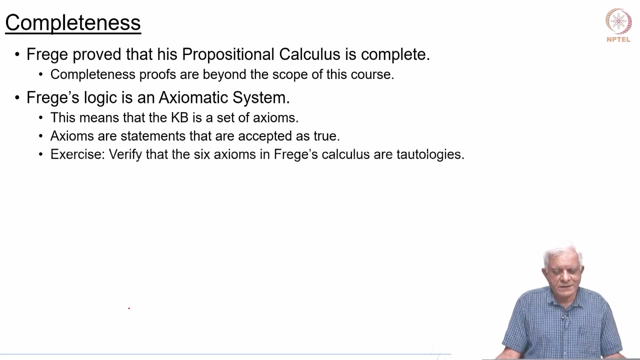 that false will again become true essentially. So they are equivalent essentially. Why do we need these things, which are sometimes obvious? because the proof system is a formal system, a. This is a statement which is always true. essentially, It is a sentence. it can be a compound sentence. 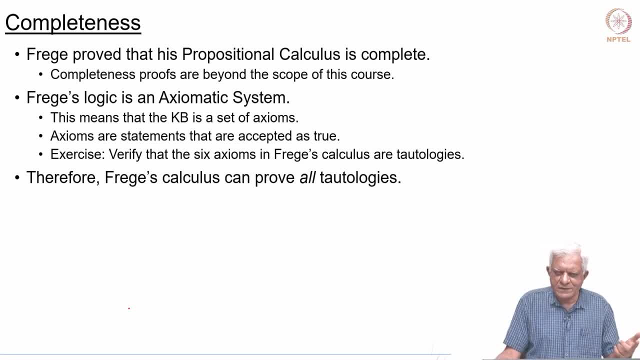 it cannot be a simple sentence because, unless you use a particular symbol, which we will see when we look at the first logic that we are looking at, So, essentially, what this says is that you have started off with a set of statements which are known to be true. 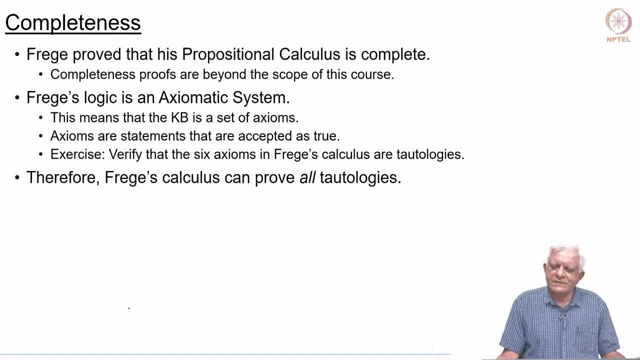 And then you can, it is complete. so you can derive all entailed statements. So all entailed statements also must be true. So in other words, we can derive all tautologies essentially, and by tautology again we mean statements which are true By the way we have talked. 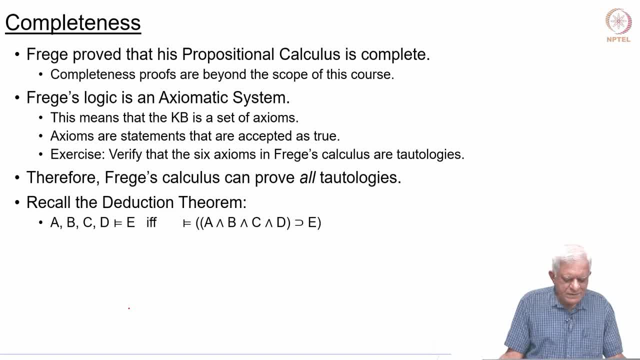 about the deduction theorem. it said that z découv calendrico, ale só la dedução. So if, in this example, E is entailed from A, B, C and D, then this is equivalent to saying that if you construct a formula, which is, which has all the antecedents joined together, 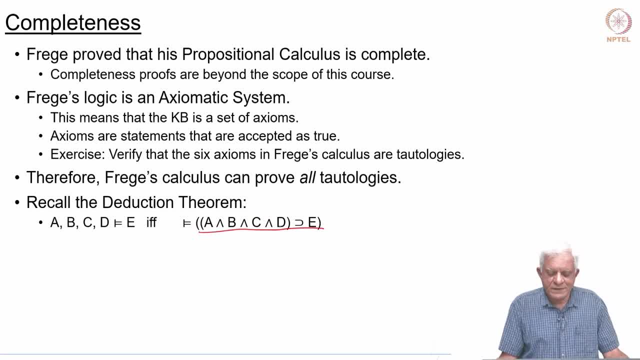 by, and so A and B and C and D, and then you put this implies E. these two are logically equivalent. The deduction theorem says that if given A, B, C, D, you can show E. it is equivalent to saying that you can show that A and B and C and D implies E. essentially we will revisit. 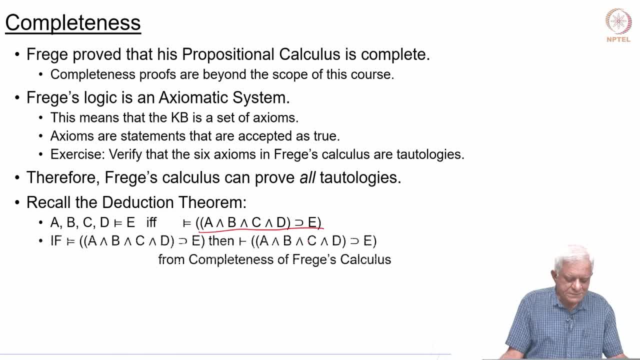 this and we will revisit the use of this also. But if the thing which I have underlined is true, which means so what is the why? is this a tautology? Because this is the empty there is. this is empty. there is nothing there. 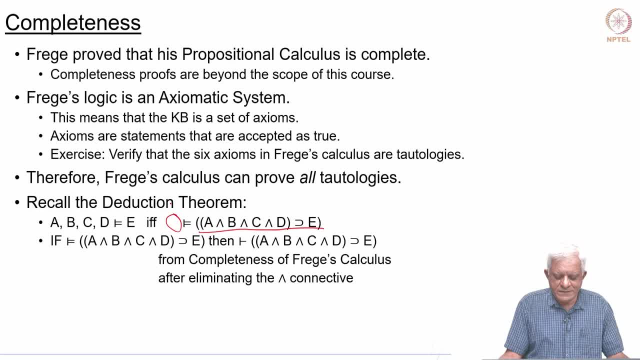 You do not need anything to be able to show that A and B and C and D, the whole thing implies E. You can show that it is true essentially. you know that it is true. it is entailed by nothing, essentially. So it is true. it stands by itself. 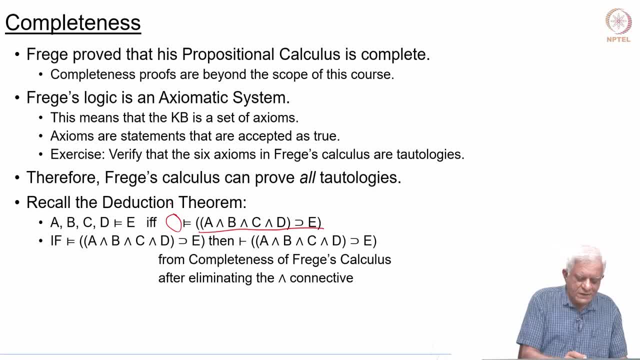 Now go, since Frege's system is complete. we know that if this is the tautology or which is which can be Can be derived from nothing, then you should be able to derive this as as well as we should be able to derive. 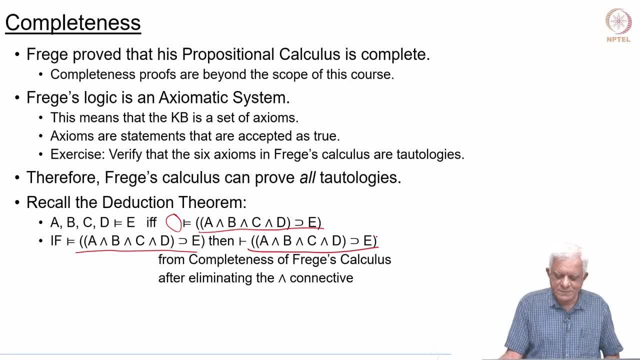 So if it is entailed, then it can be derived. that is what completeness means, right? So if you can derive this out of nothing, that means if you were given A, B, C, D, then you could have derived E. essentially, 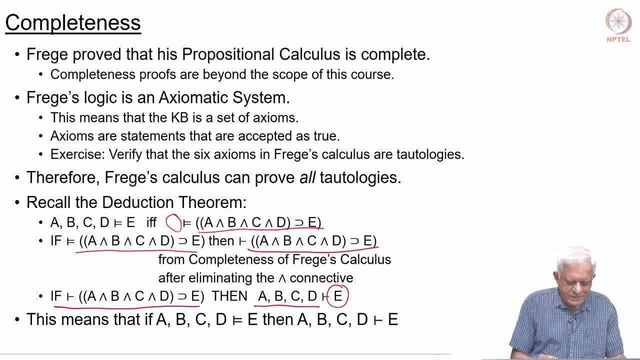 Ok. So if you now connect this first thing and the last thing, the first thing was what A, B, C, D, E entails E. Now we are shown that, given this A, B, C, D E, we can derive E. 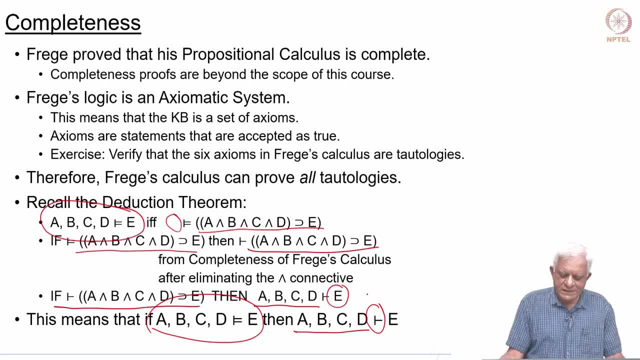 So remember the difference between derivation and entailment. essentially So, this means that not only is Frege- Yes, Yes, Yes, Yes- is system powerful enough to derive all tautologies, The fact that you can derive all tautologies. 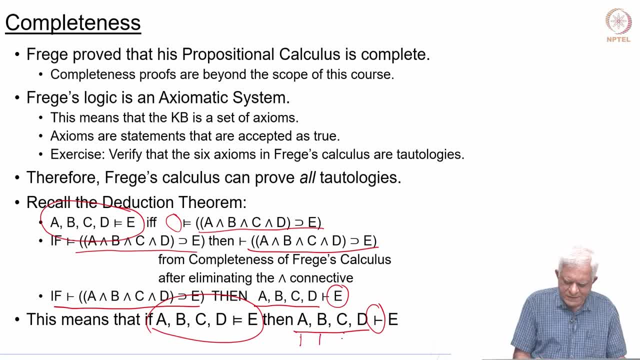 means that if you are given some premises, for example A, B, C, D, somebody has told you that these are true, and then if E is entailed from those premises, then you can also derive it. So in that sense the logic is complete. 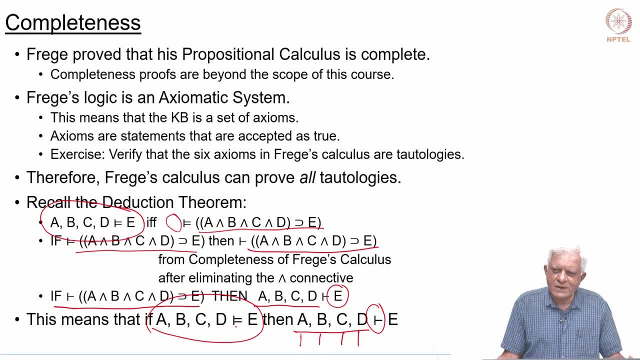 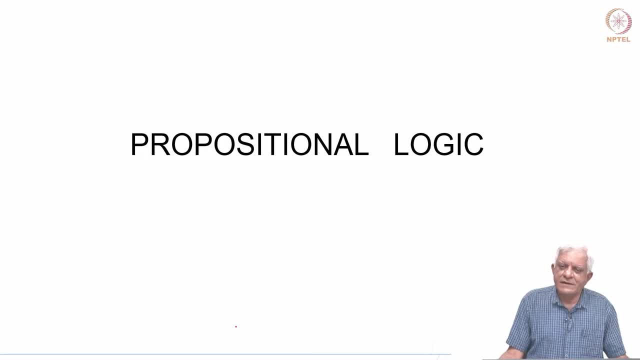 So now it is time to look at our first language. We shall do that after a short break. Think about the notion of completeness, of set of expressive, set of connectives, and also the notion of completeness in terms of being able to derive all true statements. And then we 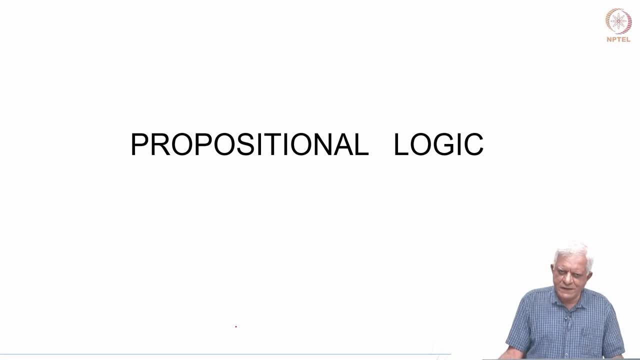 will now move to a specific logic language. We have not defined a language so far. We have said that alpha, beta, gamma are some sentences in some language, but now we are going to define a language, and that language is the simplest of all languages. called proportional logic. We will do that after this short break.